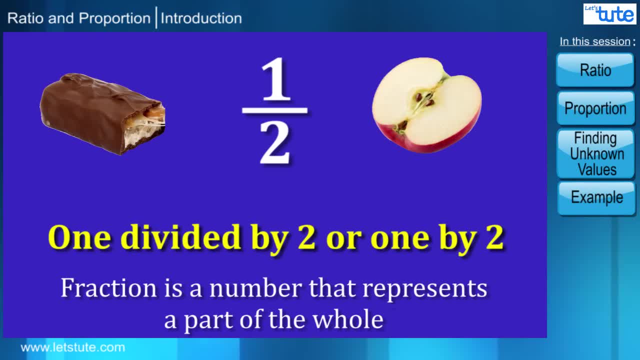 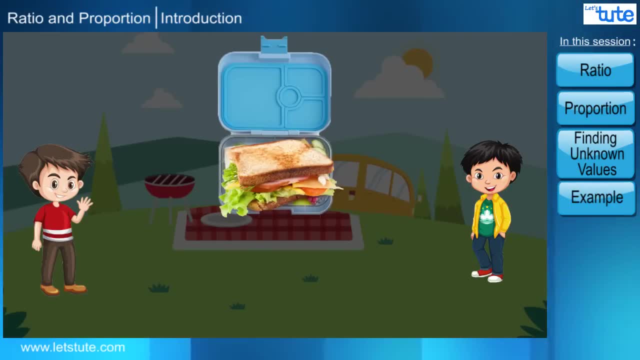 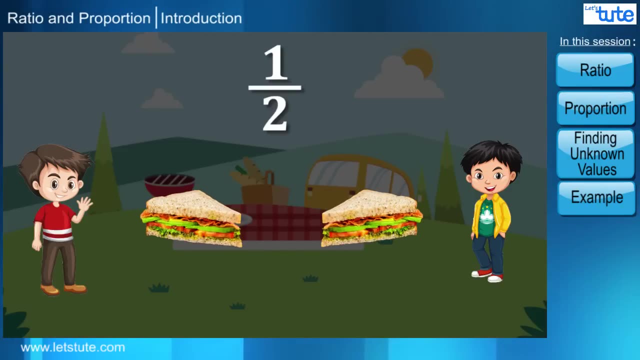 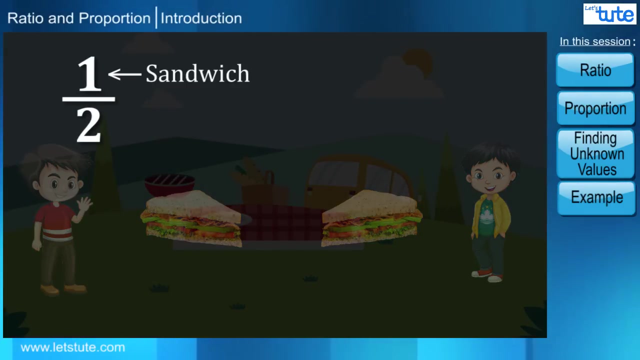 Well, let me tell you one more interesting thing about this number. If you go to a picnic and two of your friends have to share one sandwich, Then how much will one of the friends get Half of the sandwich? right, And this is a fraction, like we said before. Or we can also say that one sandwich is shared between two people. 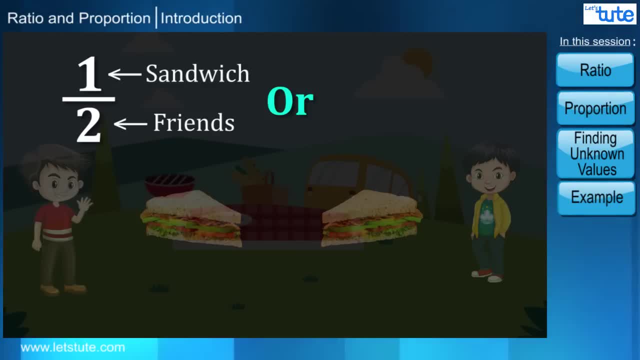 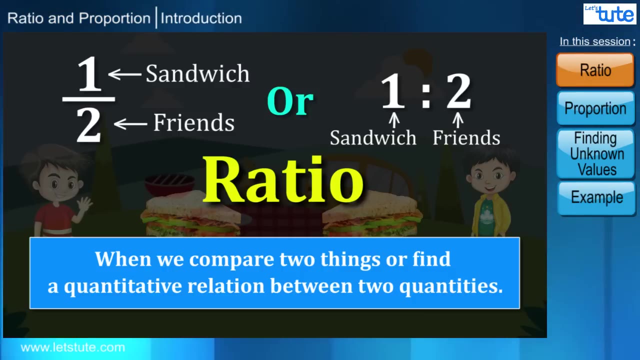 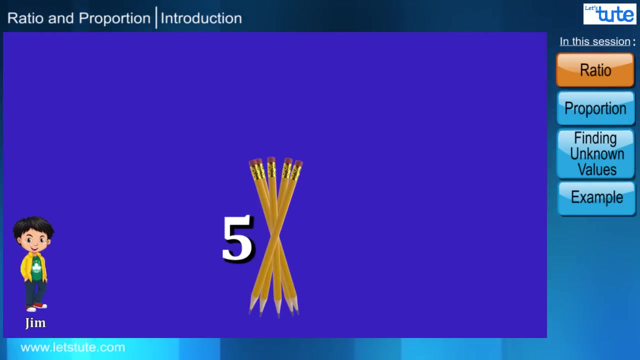 That is 1 divided by 2, or 1 is to 2.. And numbers in this form are known as ratio. When we compare two things or find a quantity, we can say that it's a ratio. In the quantitative relationship between two quantities we get ratios. For example, 5 pencils are to be divided between two friends, Jim and Tim. in the ratio of 3 is to 2 or 3 by 2.. 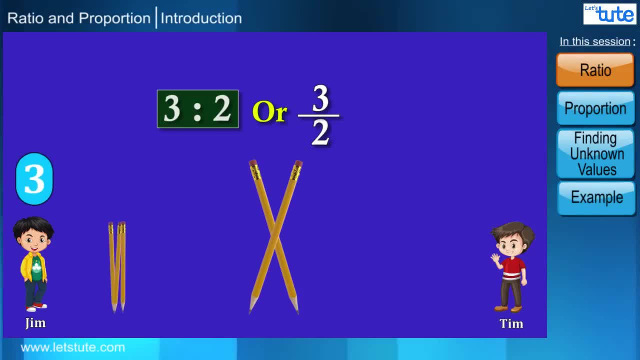 This means we will have to give 3 pencils to Jim and 2 pencils to Tim, correct? But here is 3 by 2. the fraction No Here. the fraction of pencils to Jim is 3 by 5 and to Tim is 2 by 5, ie, you have. 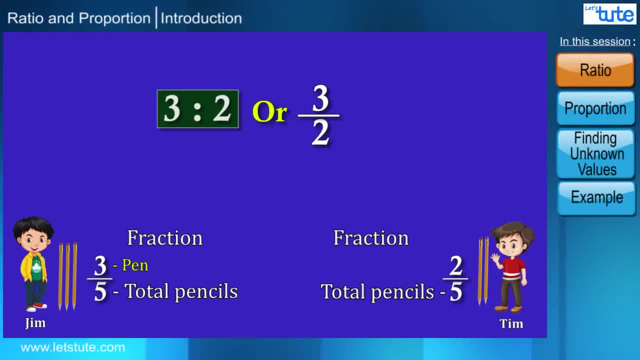 total 5 pencils and out of that 3 pencils you have given to Jim And out of 5 pencils you have given 2 pencils to Tim. But in the ratio where it says 3 is to 2 or 3 divided, 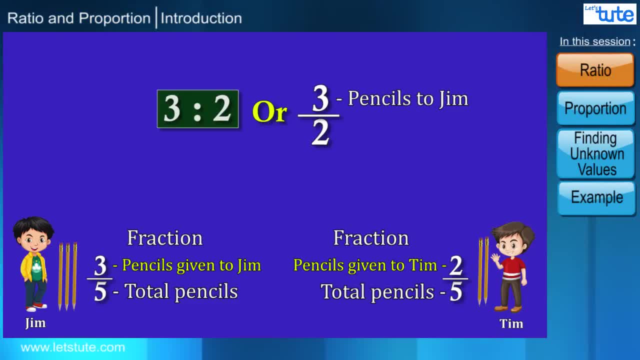 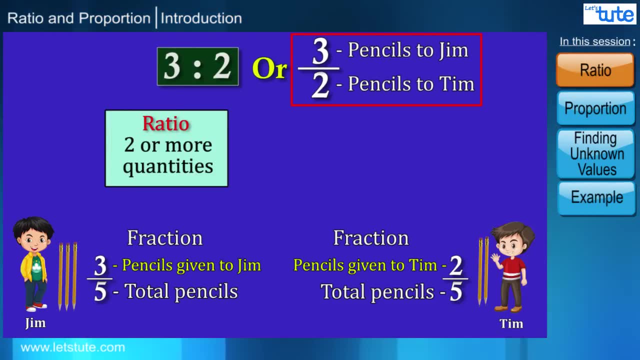 by 2. It means you have to give 3 pencils to Jim and 2 pencils to Tim. Ratio deals with 2 or more different things or quantities, whereas fraction deals with only one quantity. I hope this difference between ratio and fraction is clear. now Let's continue. the same example. 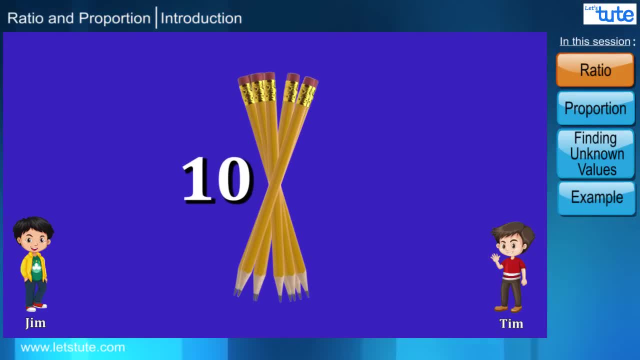 of Jim and Tim. Now suppose if there are 10 pencils to be divided between Jim and Tim, in the ratio of 3 is to 2.. How will we do this Now? Jim will get 3 pencils and Tim will get 2 pencils. We are still left with 5 pencils, So we will repeat the procedure, that is 3. 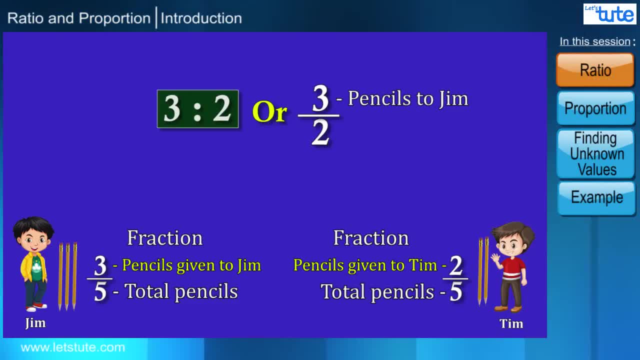 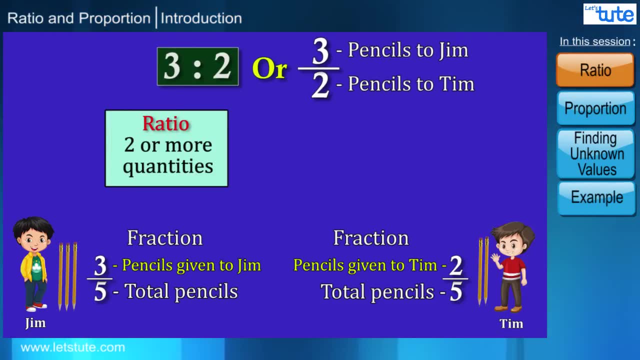 two. It means you have to give three pencils to Jim and two pencils to Tim. Ratio deals with two or more different things, or quantities, whereas fraction deals with only one quantity. I hope this difference between ratio and fraction is clear. now Let's continue. the same example of 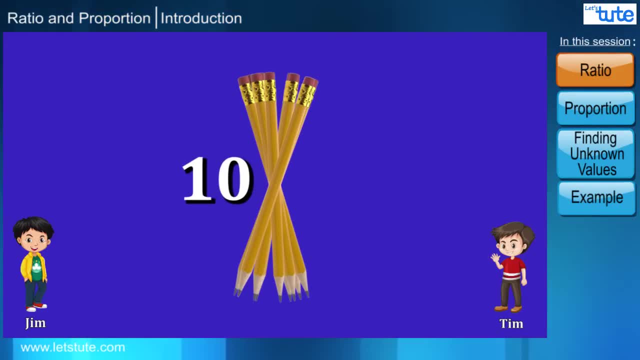 Jim and Tim. Now suppose if there are 10 pencils to be divided between Jim and Tim in the ratio of 3s to 2.. How will we do this? Now? Jim will get three pencils and Tim will get two pencils. We are still left with five pencils, So we'll repeat the procedure, that is, three pencils to Jim and two. 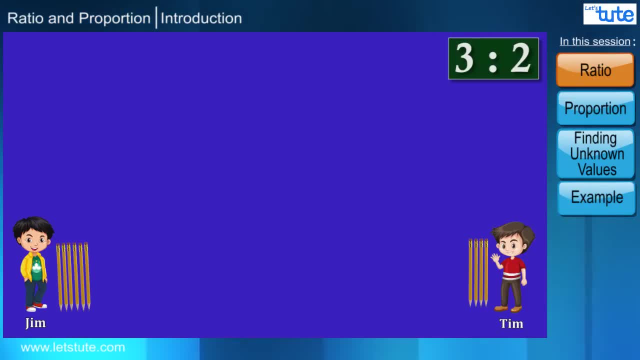 pencils to Tim. Well, now, in total Jim has six pencils and Tim has four pencils, or their ratios of pencils is six, So we can write this as 3s to 4 or 6 by 4.. But wait, we were given that pencils should be divided in the ratio of 3s to 2.. 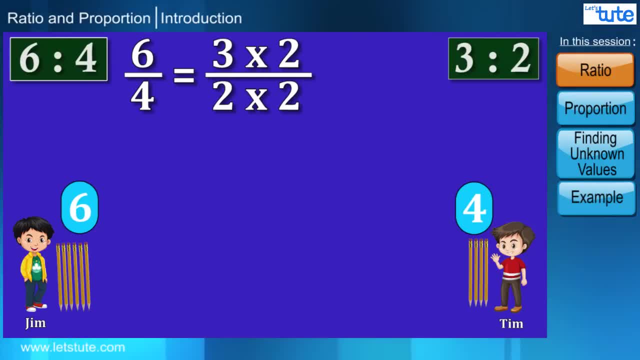 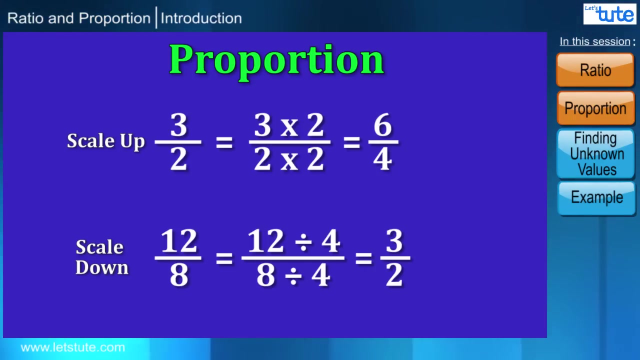 You can write this as now we can cancel 2 and we will get 3 by 2 only, which means 3s to 2 is equal to 6s to 4.. And this is known as proportion. So if we scale up or scale down a ratio, that is, multiply or divide the numerator and denominator by the same number, 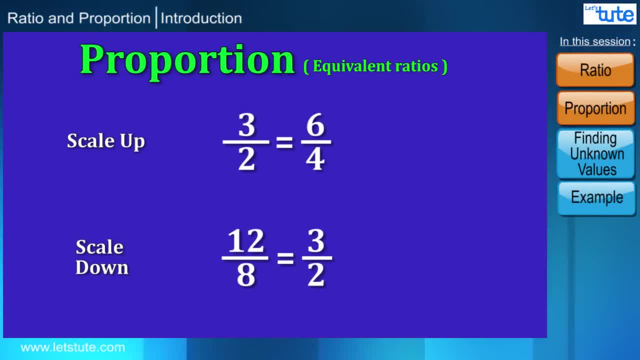 We will get ratios which are equivalent, that is, equivalent ratios, and proportion is nothing but equivalent ratios. Here, 6s to 4 is equal to 6s to 4.. Here, 4s to 4 is equal to 6s to 4.. Here, 3s to 4 is equal to 6s to 4.. Here, 3s to 4 is equal to 6s to 4.. Here, 3s to 4 is equal to 6s to 4.. 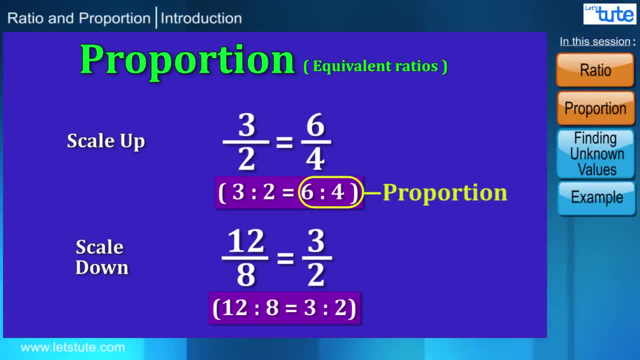 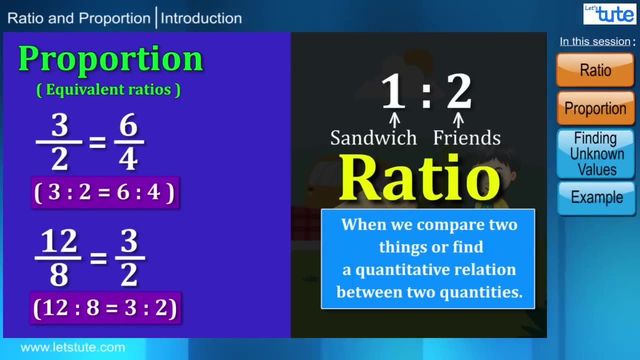 is a proportion of the ratio: 3 is to 2.. Similarly, for 12 is to 8,, 3 is to 2 is also a proportion. Now we know what is ratios and what is proportion right, And also the difference between them. 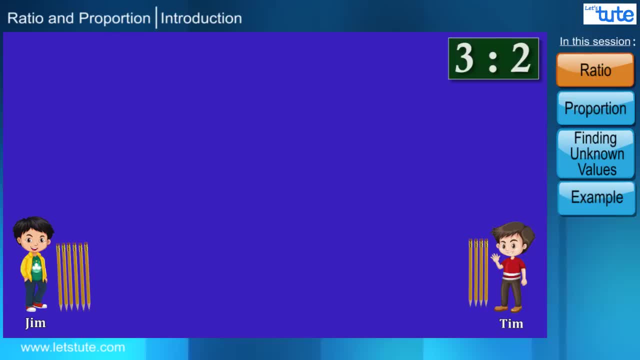 pencils to Jim and 2 pencils to Tim. Well, now, in total, Jim has 6 pencils and Tim has 4 pencils, or their ratios of pencils is 1.. 6 is to 4 or 6 by 4.. But wait, We were given that pencils should be divided in the ratio. 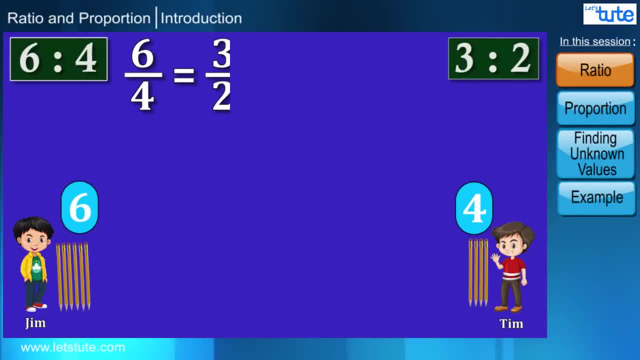 of 3 is to 2.. You can write this as Now: we can cancel 2 and we will get 3 by 2 only, Which means 3 is to 2 is equal to 6 is to 4. And this is known as proportion. 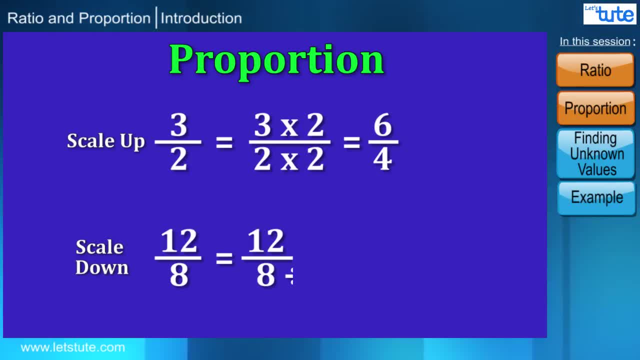 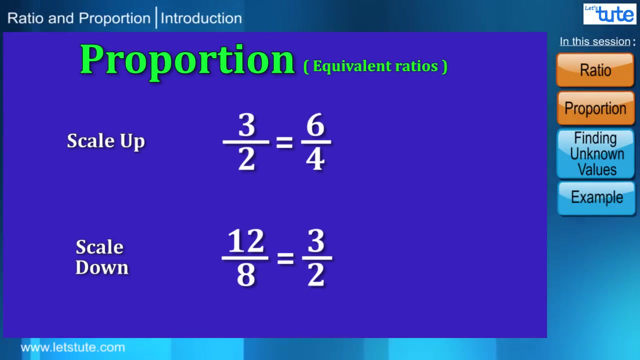 When we scale up or scale down a ratio, that is, multiply or divide the numerator and denominator by the same number, We will get ratios which are equivalent. that is, equivalent ratios And proportion is nothing but equivalent ratios. Here, 6 is to 4 is a proportion of the ratio. 3 is to 2.. Similarly, for 12 is to 8.. 3 is to 2. 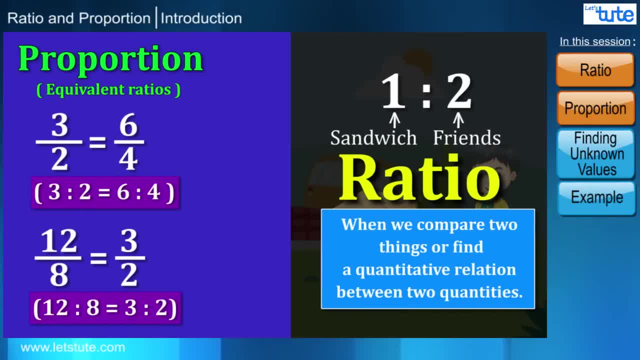 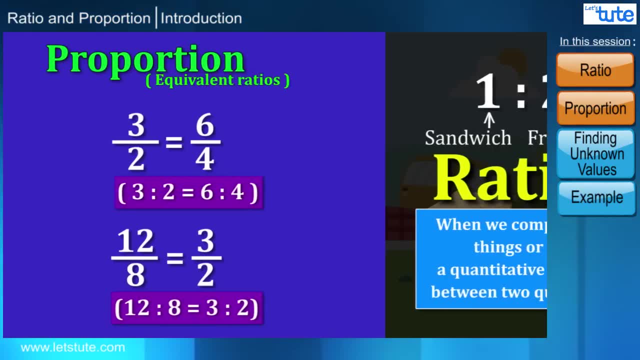 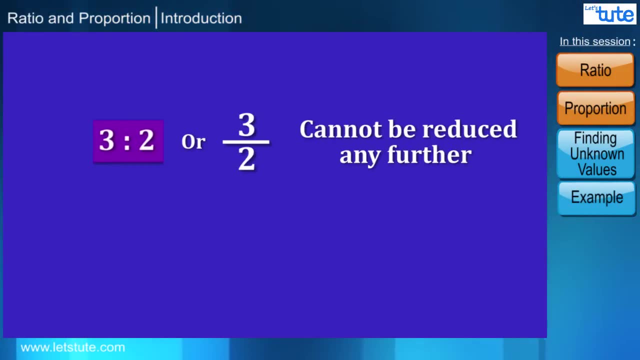 is also a proportion. Now we know what is ratios and what is proportion- Right, And also the difference between them. Here, when we look at the same example, 3 is to 2 cannot be reduced any further, Right, So when a ratio cannot be reduced. 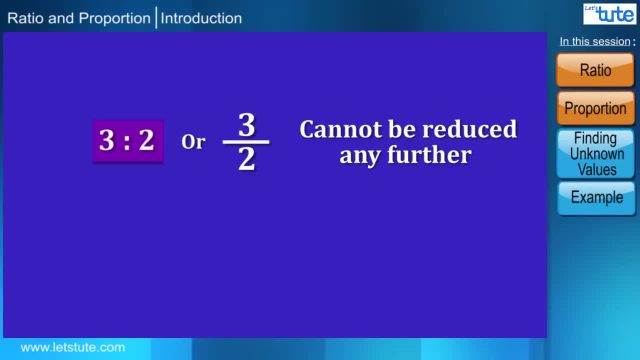 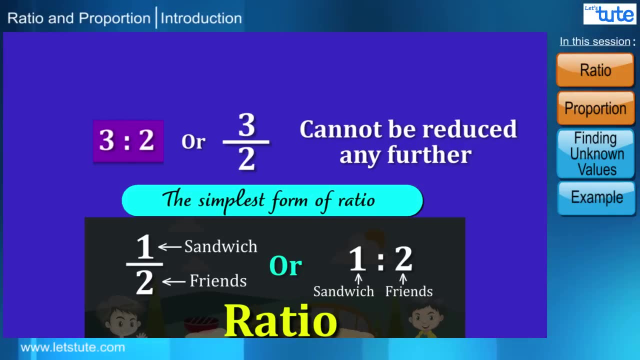 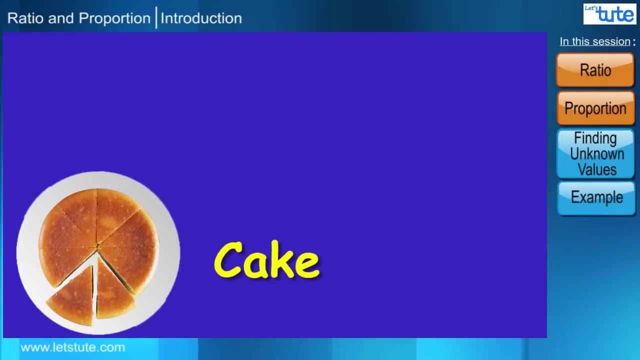 Then it is known as the simplest form of ratio. However, the concept of ratio and proportion is not based on just 2 quantities. For example, if you are making a cake, Then for that you will need 2 bowls of flour, 1 bowl of butter and 3 bowls of sugar. Here the ratio of flour. 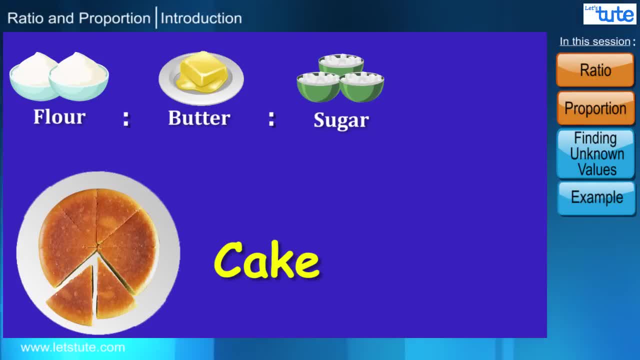 to butter to sugar can be written as 2.. Here the ratio of flour to butter to sugar can be written as 2.. can be written as 2 is to 1 is to 3.. Here the order plays a very important role. 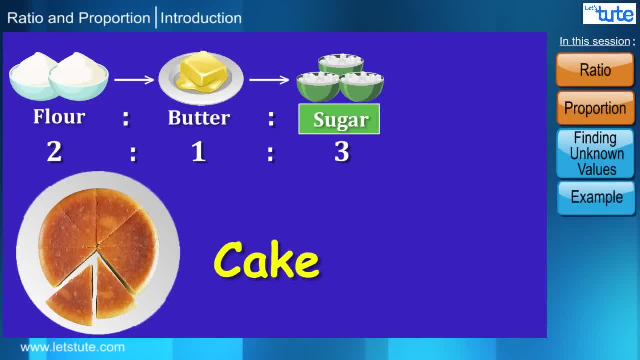 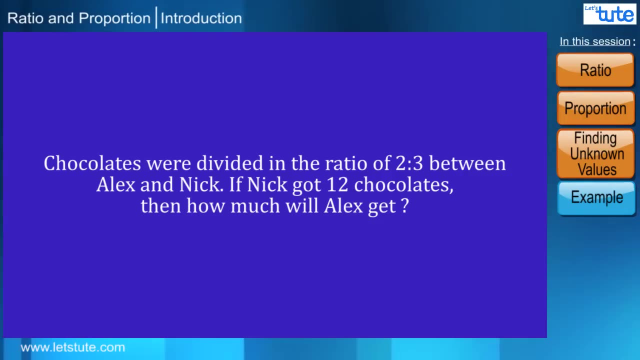 This can also be further extended to four quantities. also, like you can add a bowl of chocolate too. Proportions are also used to find unknown quantities. For example, chocolates were divided in the ratio of 2 is to 3 between Alex and Nick. If Nick got 12 chocolates, 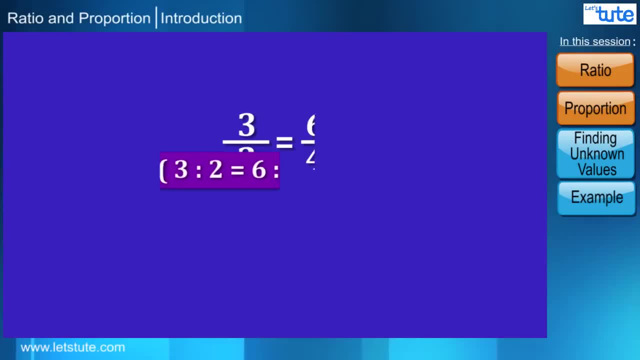 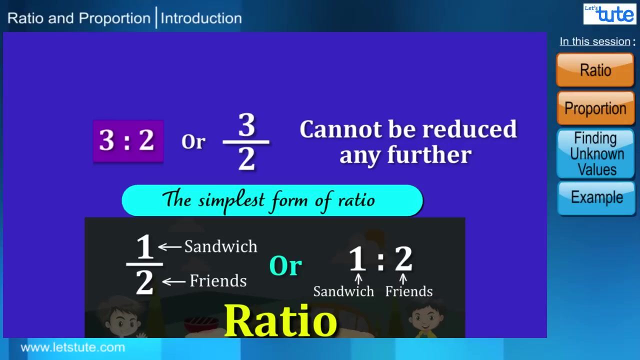 Here, when we look at the same example, 3 is to. 2 cannot be reduced any further, right? So when a ratio cannot be reduced any further, then it is known as the simplest form of ratio. However, the concept of ratio and proportion is not based on just two quantities, For example. 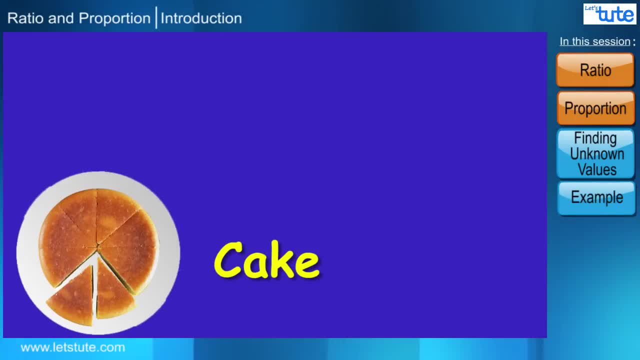 if you are making a cake, then for that you will need 2 bowls of flour, 1 bowl of butter and 3 bowls of sugar. Here the ratio of flour to butter, to sugar can be reduced. So when a ratio cannot be reduced any further, then it is known as the simplest form. 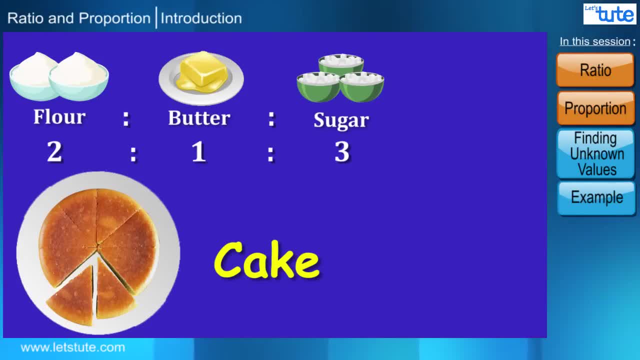 written as 2 is to 1 is to 3.. Here the order plays a very important role. This can also be further extended to 4 quantities. also, Like you, can add a bowl of chocolate too. Proportions are also used to find unknown quantities. For example, chocolates were divided in the ratio of 2 is to 3. 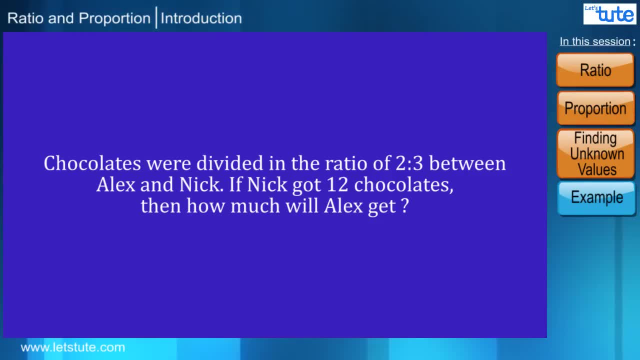 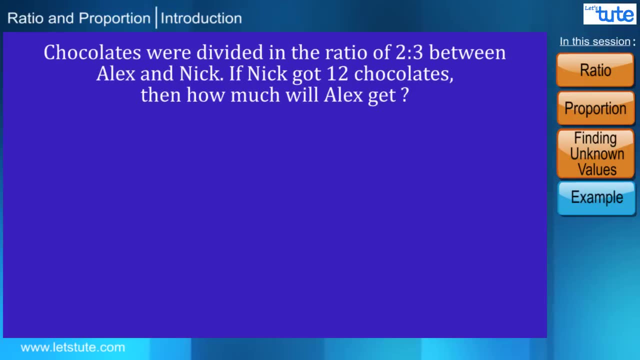 between Alex and Nick. If Nick got 12 chocolates, then how many chocolates did Alex get Here? we know the ratio of chocolates between Alex and Nick is 2 is to 3. And we can write this as now we know Nick has got 12 chocolates, So let's put. 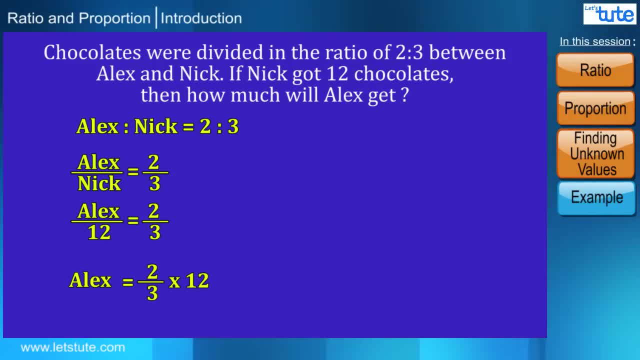 that value here. After cross-multiplying we get the value as 8.. That is, Alex will have 8 chocolates. Proportions are majorly used in such cases where we have to find out the ratio of chocolate in the unknown values. Well, I hope now you guys are completely clear that what is a fraction? 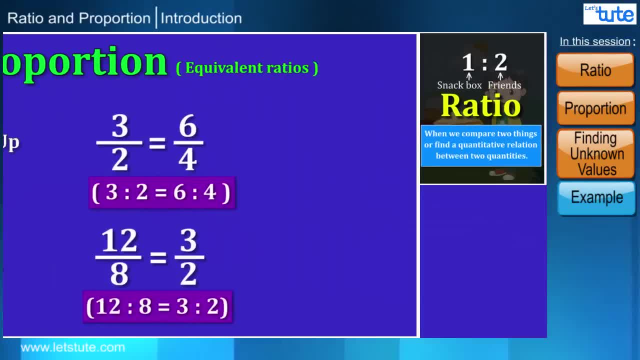 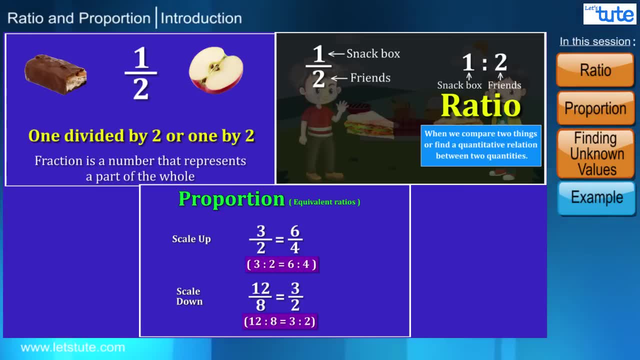 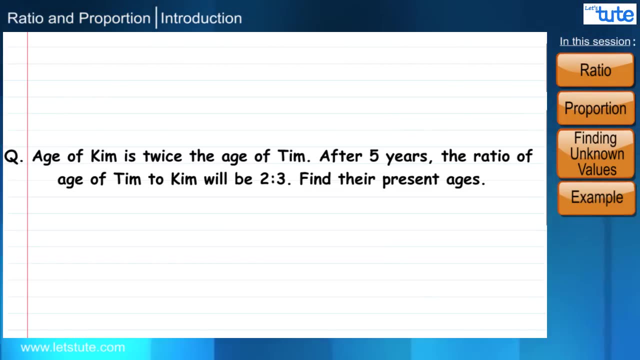 what is a ratio and what is proportion, and also the difference between all the three. Let's look at a little complicated problem before we end this session. If the age of Kim is twice the age of Tim after 5 years, the ratio of age of Tim to Kim will be 2 is to 3.. Find their present. 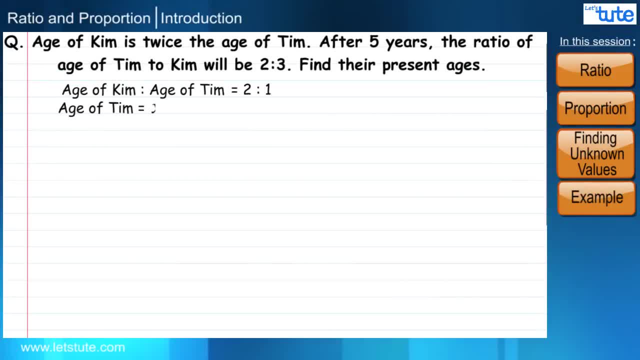 age. If the age of Tim is twice the age of Tim, after 5 years the ratio of age of Tim to Kim will be 2 is to 3. Find their present age. Here we can consider the age of Tim as X. and since it is said that the age of Kim 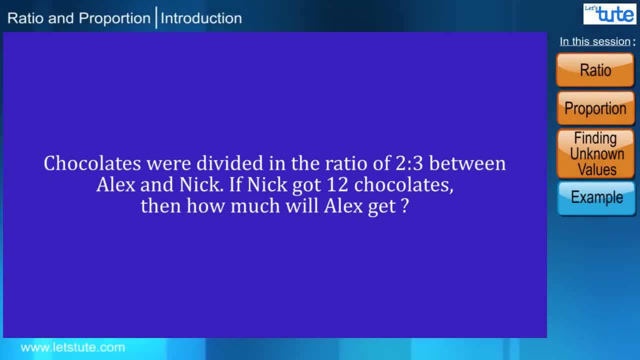 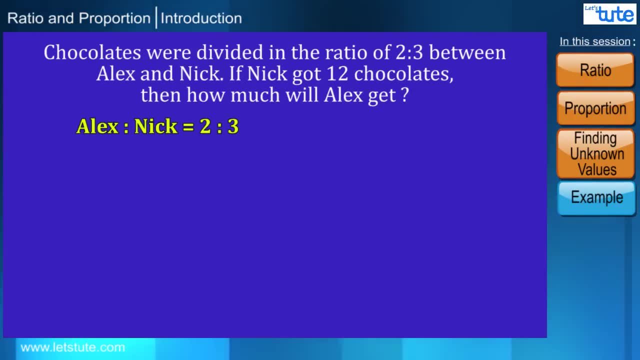 then how many chocolates did Alex get Here? we know the ratio of chocolates between Alex and Nick is 2 is to 3, and we can write this as now we know Nick has got 12 chocolates, so let's put that value here. After cross-multiplying, we get the value as 8,. 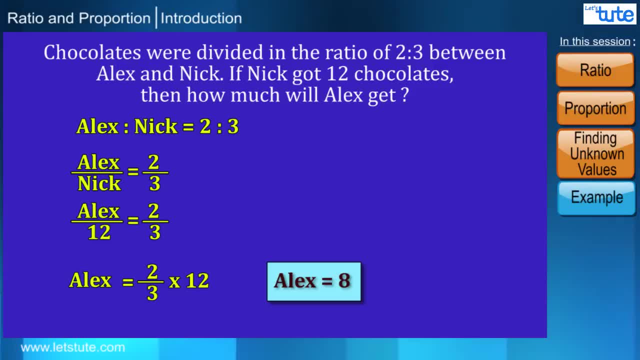 that is, Alex will have 8 chocolates. Proportions are majorly used in such cases where we have to find unknown quantities Here. we know the ratio of chocolates between Alex and Nick is 2 is to 3, that is, Alex will have 8 chocolates. Proportions are majorly used in such cases where we have to find 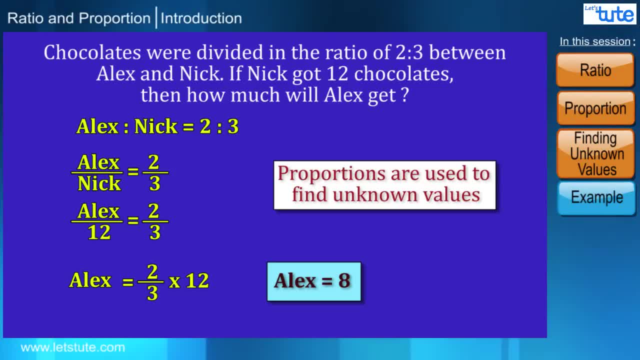 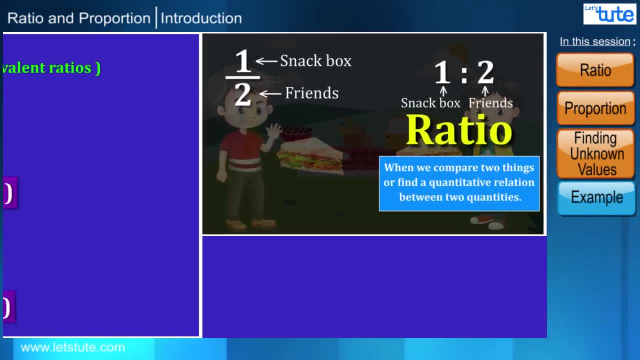 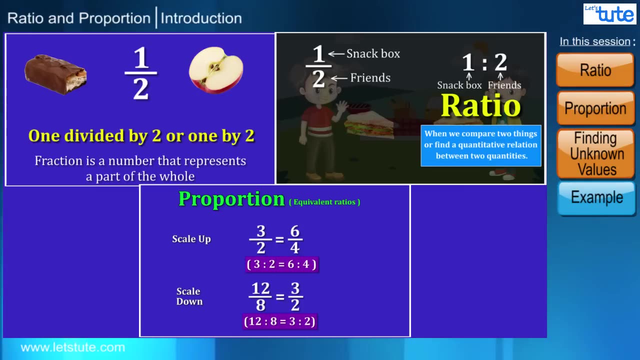 the unknown values. Well, I hope now you guys are completely clear that what is a fraction, what is a ratio and what is proportion, and also the difference between all the three. Let's look at a little complicated problem before we end this session. If the age of Kim is twice, 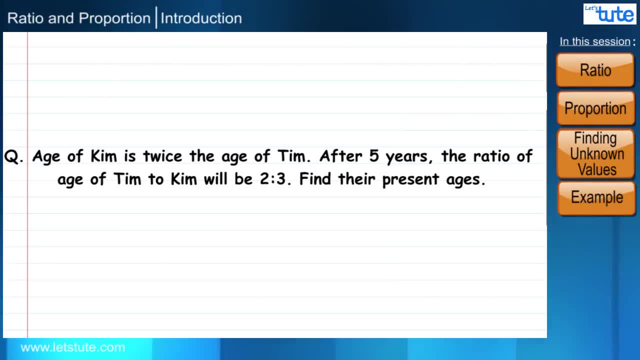 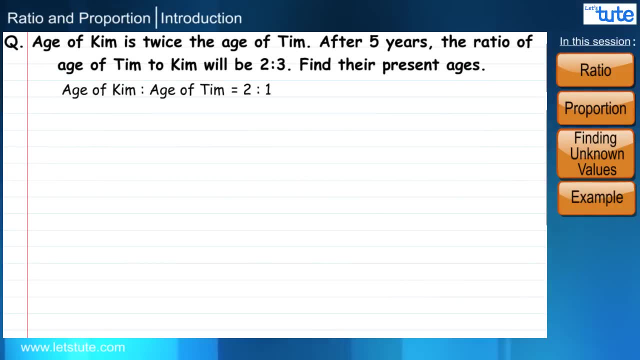 the age of Tim. after 5 years the ratio of age of Tim to Kim will be 2 is to 3.. Find their present ages. here we can consider the age of Tim as X, and since it is said that the age of Kim is twice, 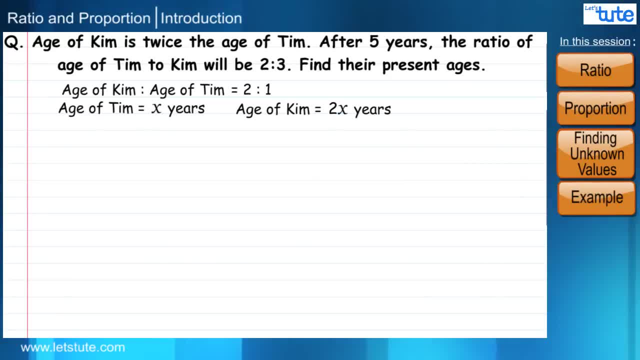 the age of Tim. we will write it as two X correct. Next, it is that after five years the ratio of the ages is 2 is to three. So after five years the age of Tim will be X plus five and age of Kim will be 2X plus. 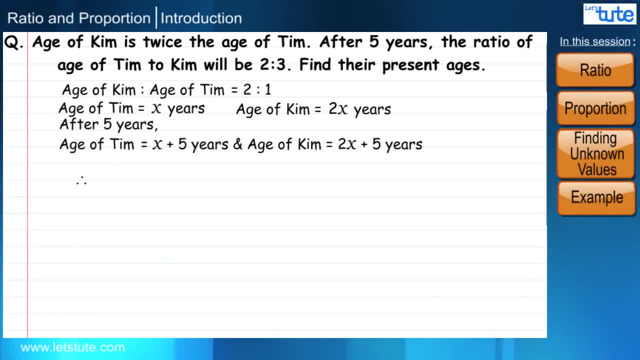 and their ratio. that is x plus 5 divided by 2x plus 5 is equal to 2 is to 3, that is, 2 by 3. after cross multiplying, we will get the value of X as 5 years. hence the age of Tim is 5 years and Kim's age is twice the age of Tim, which will be 10. 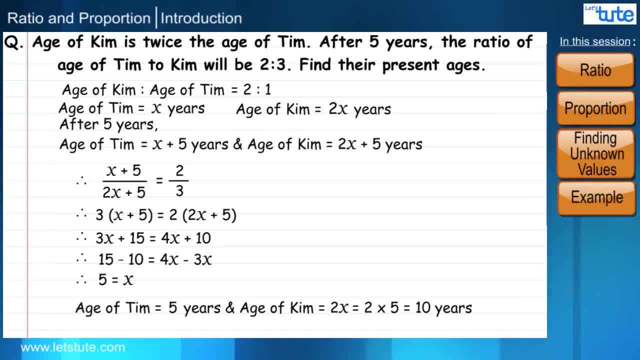 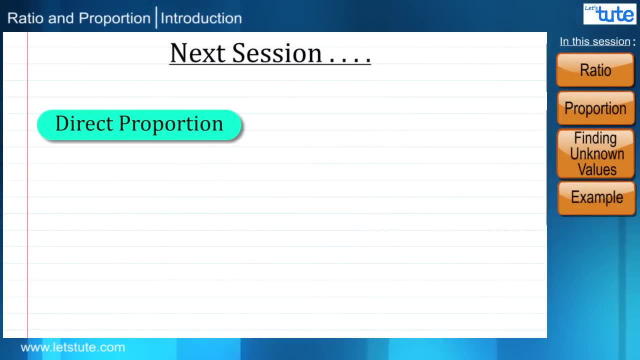 years. we can also cross check this by putting the values of x in this equation to see if we get the ratio as 2 by 3 or not. let's check that. well, that's it for today's session. in our next session we will see what is direct.